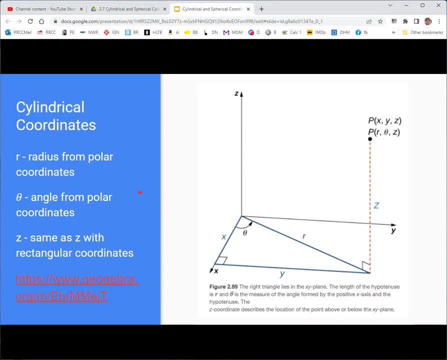 So that should be helpful, that if you know polar coordinates then you know these three coordinates that you're switching and even the formulas we'll use to get between them. We see a general point here, in three-dimensional space of course, given by x, y and z. 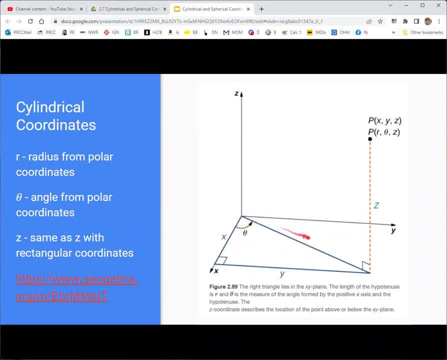 but you can also get to it using r and theta and that'll get to that spot in the x- y plane. and then you go up with z in the same way And there's a little link here to go to a GeoGebra interactive. 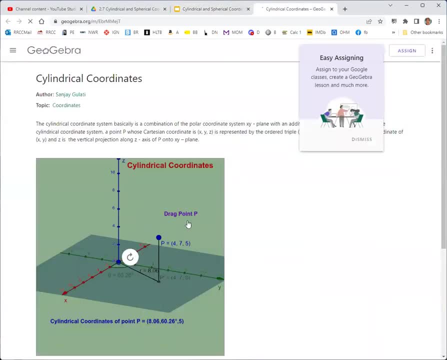 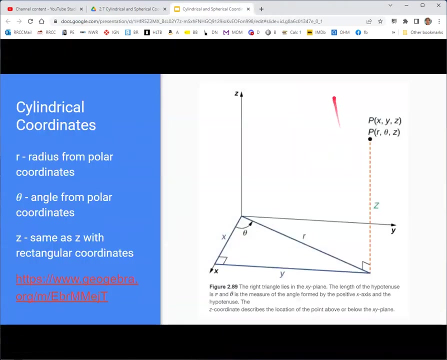 thing to play around with the cylindrical coordinates And so you can drag this point around and see how the coordinates change in cylindrical coordinates. So feel free to interact with that. Now the formulas for converting: of course, z is equal to z, and then these are your polar. 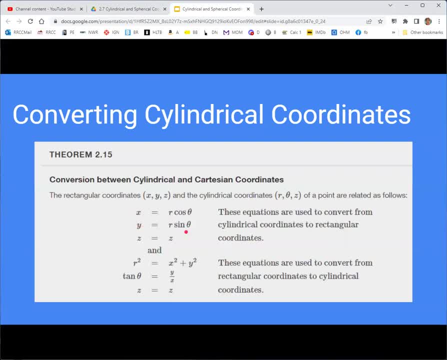 coordinate formulas: x is r cosine theta, y is r sine theta. So if you had r theta z, you could use these to get x, y and z. If you have x, y and z and you need to get r, 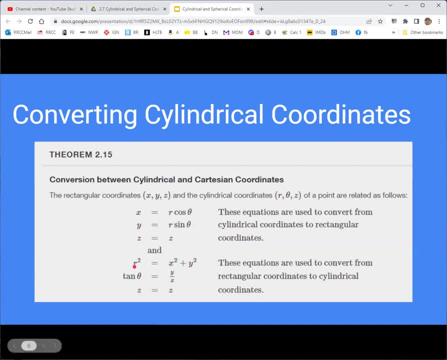 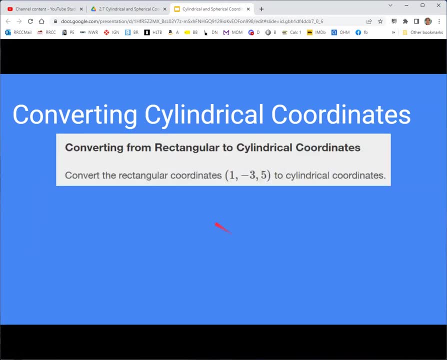 theta z. well, z is still the same and we would use the Pythagorean theorem to get r and then tangent to get theta. So let's say you were converting from rectangular coordinates- one negative three, five, to the cylindrical coordinates. You would start by maybe saying: 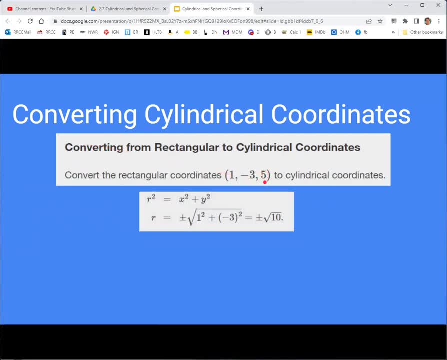 z is still equal to five. right, Because that doesn't change. But then to get r you would use the square root of the sum of the squares of those first two components, And we always use the positive r for this, because r is supposed to be a radius, So we'd use positive. 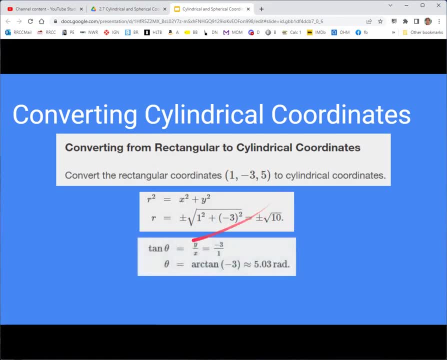 square root of 10 here. And then tangent of theta would be y over x, So that's negative three over y. And then tangent of theta would be y over x, So that's negative three over y. And then tangent of theta would be y over x, So that's negative three over y. And then 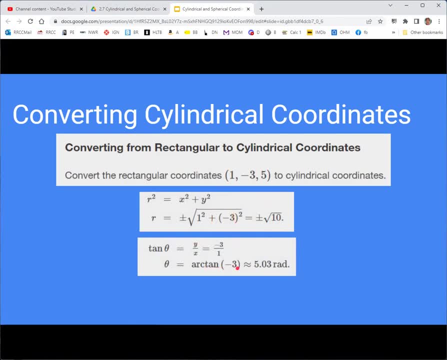 the inverse tangent And you want theta restricted to zero over two pi Again with the calculator. sometimes this inverse tangent on your calculator will give you a negative angle. You want to convert that to the equivalent positive angle. coterminal positive angle. 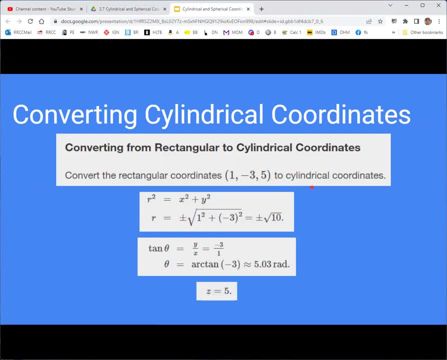 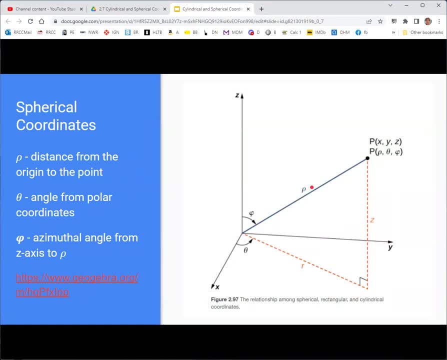 Again, z should be the same. There's an example converting rectangular to cylindrical. Now talk a little bit about spherical coordinates. Their rho, the Greek letter rho. it's not a p, It just looks kind of like a p. Greek letter: rho. Greek letter theta. 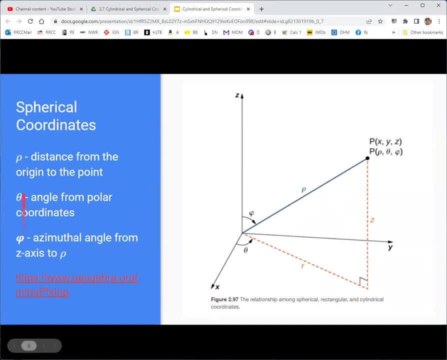 and Greek letter phi. So rho, theta and phi, And theta is the same, theta from cylindrical coordinates and polar coordinates. So that's the one thing you already know. Rho is pretty easy to understand. It's sort of a three-dimensional radius. So go straight from the origin to 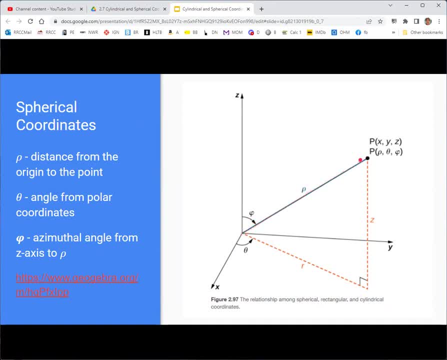 the point that shortest distance along that straight line And that's rho, So that should also be positive. And then phi is the azimuthal angle. So if you think of starting in the positive z direction and then drawing down towards the xy plane, 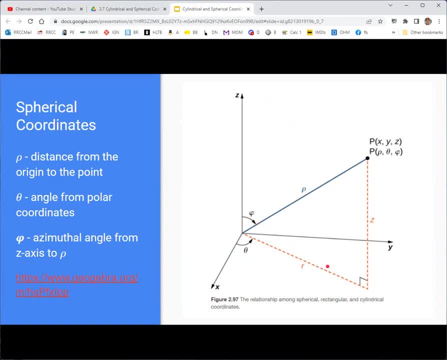 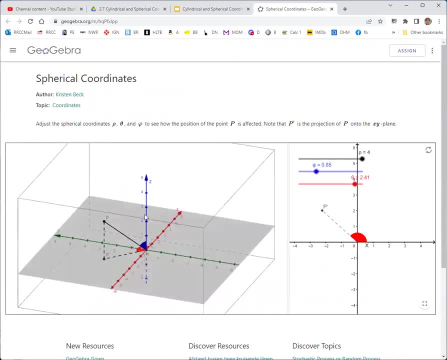 that will give you your phi Again. there's an interactive here so that you can mess around with changing this In this one. you can change that there And you change r, Though some people do work with negative rho values. So this one does negative rho values, but we're going to try to use positive And then you could. 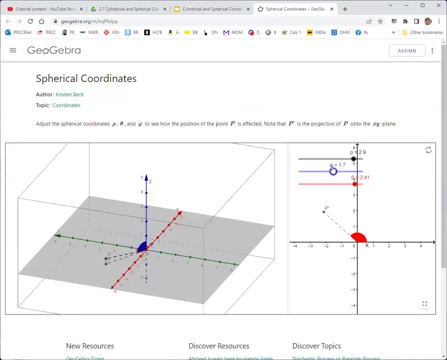 see the effect of changing phi. So if phi hits pi over 2, you're at the xy plane. So phi only goes from 0 when it's at the positive z, and then it's pi or 180 when it's at the negative z. 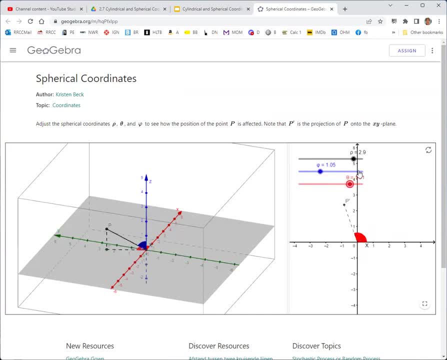 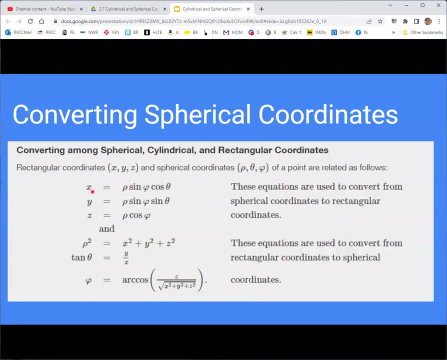 And then of course, theta is the normal theta that just sweeps around 0 to 2 pi. Here's the equations that relate the two. We basically take the equations from cylindrical and replace r with rho sine v, And that gives you your xy equations. And then z is rho cosine v. 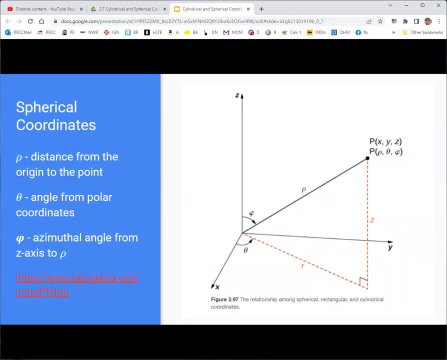 And then you can actually see that from here, because you can just draw right triangle here And this is also z, which rho is the hypotenuse. So that's rho cosine v as the adjacent side, And then r- this is also r up here- That's rho sine v. So just using that, 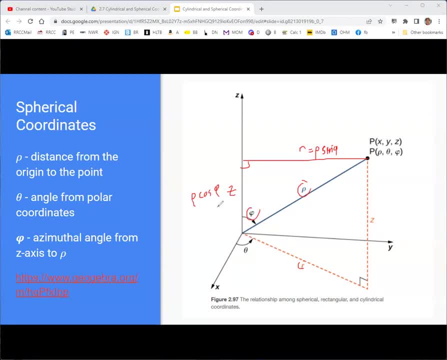 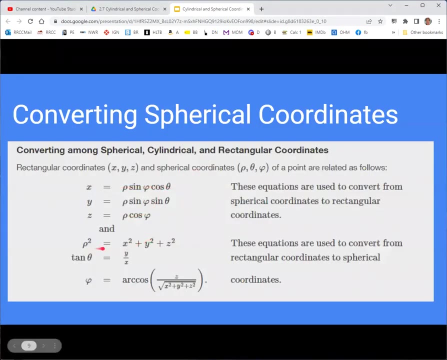 right triangle. there, with phi as your angle and rho as your hypotenuse, you can get the relationship between rho and v and r and z. So that gives you these equations: Rho in terms of x, y and z is just the three-dimensional. 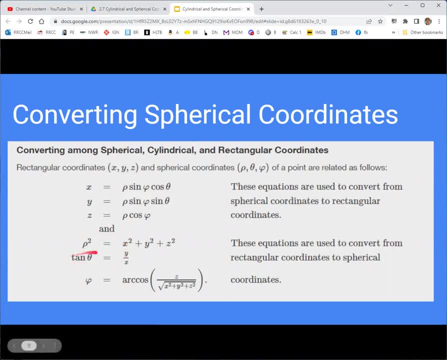 distance equation. And then remember, theta is the same theta, So tangent of theta is still y over x. And then this one looks complicated, but it's really just inverting this equation, Solving for phi. here you'd have: phi is inverse cosine of z over rho And they've replaced rho. 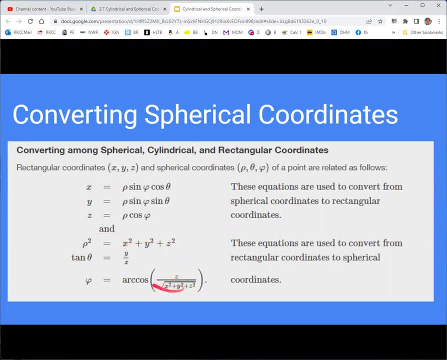 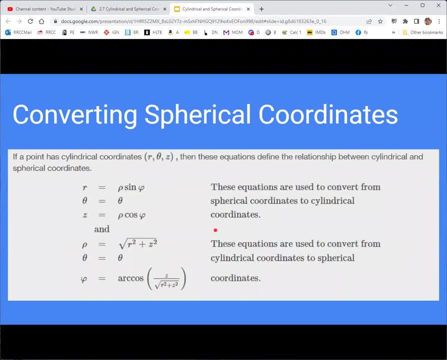 with the square root of the sum of the squares from this one, So that you just use x, y and z. But this is just inverse cosine of z over rho. If you want to go between cylindrical and spherical directly, you can, though most people just go to rectangular. It's kind of a middle step. 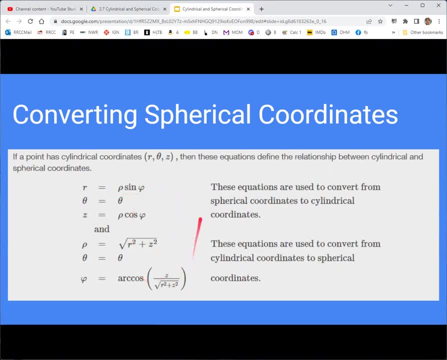 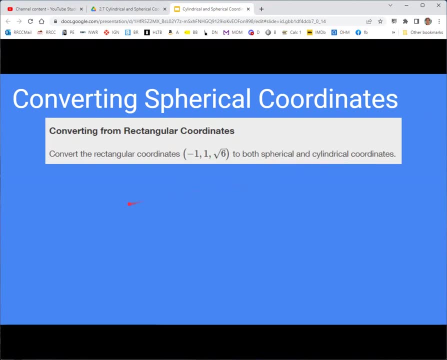 rather than remembering these. But you could, if you remember those relationships there, All right, So say, I had some rectangular coordinates here and I wanted to write them as spherical and cylindrical. I think we're just going to focus on spherical here. So rho is the easy one to get. It's just the square root of the sum of the squares. 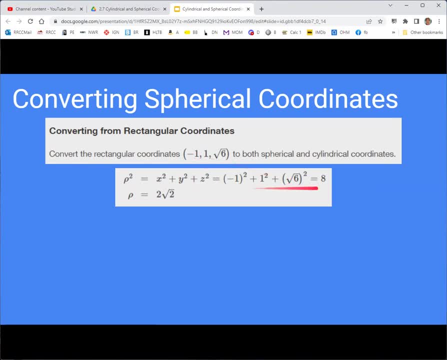 So square negative 1, square 1, square square root of 6, and you get 8.. And then the square root of 8 is 2 root, 2.. Theta is the same theta from before, And so it's inverse tangent of y over x. 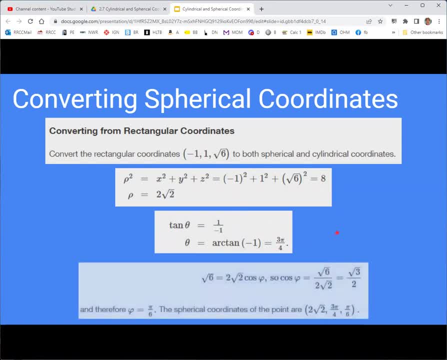 In this case it's the same theta from before, And so it's inverse tangent of y over x, And so it's 3 pi over 4.. And phi is inverse cosine of z over rho. We already have rho as 2 square root of 2.. 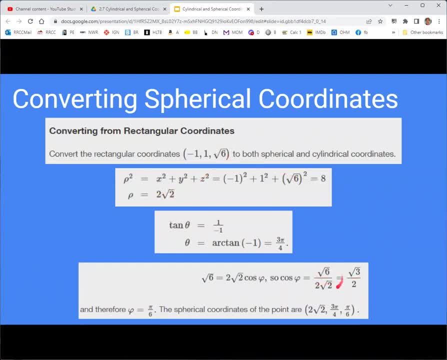 We already have z as square root of 6.. So it's just square root of 6 over 2. square root of 2 is cosine of phi. Do the inverse cosine and you get pi over 6.. So there's your spherical coordinates. 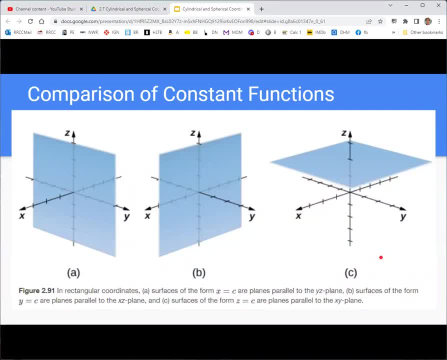 Now, if you're in rectangular coordinates, you're going to get 3 pi over 4.. And phi is inverse cosine of z over rho. We already have z over 4.. So there's your spherical coordinates And you say that x, y or z is. 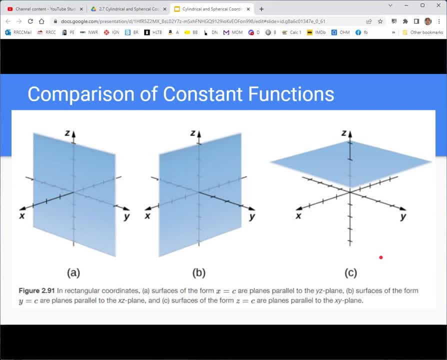 equal to a constant, you get the coordinate planes. We actually brought this up in section 2.2, I think. So it's interesting to look at when a single variable is equal to a constant for the other coordinate systems, because it's not always a plane. So if we switch over to cylindrical, 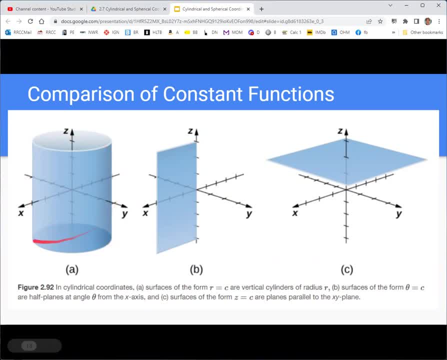 coordinates. if we let r be equal to a constant, we get the right circular cylinder. If we let theta be equal to a constant, we get a half plane. So this extends infinitely in this direction, But not in the other, And because you're restricting to positive r values. And then, if z is equal to a, 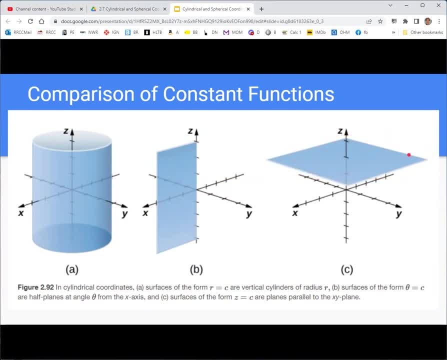 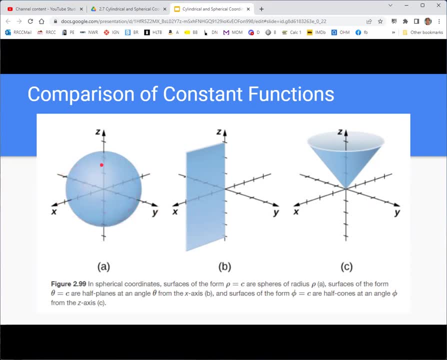 constant. that, of course, is the same, because it's the same z, from rectangular Going to spherical coordinates. if rho is a constant, you get a sphere or spheroid. If you get theta as a constant, it's the same as cylindrical, because it's the same theta. And if z is a constant, you get the top half. 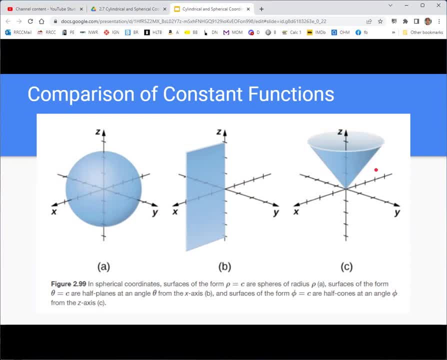 of an elliptical cone And, specifically, if you get a constant, you get a cylindrical cone And if you get a like a solid cylindrical cone, so that's v being able to a constant. very cool, uh, of course, if he was uh not acute, if it was, you know, between 90 and 180 at some obtuse angle, it would be a cone down. 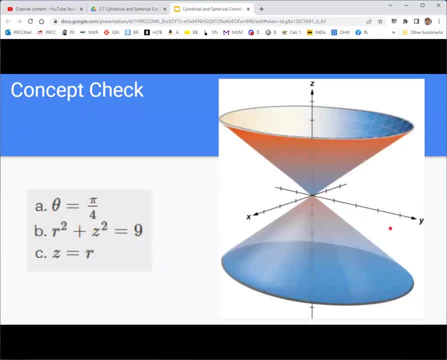 here. all right, so what if i look at this shape? uh, and i want to know what the equation is in terms of some of the coordinate systems. we looked at these quadric surfaces with rectangular coordinates, but what about using, maybe, cylindrical or spherical? so, uh, the correct answer here is c, that z is equal to r. 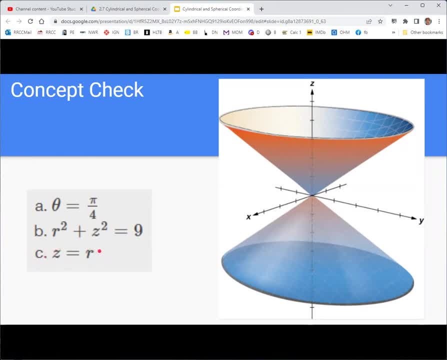 c is equal to r, then you do get the elliptical cone. and then you do get the elliptical cone, specifically the right circular cone we had as a quadric surface, and it's a much simpler equation than the rectangular coordinate equation. you notice that this line, that kind of